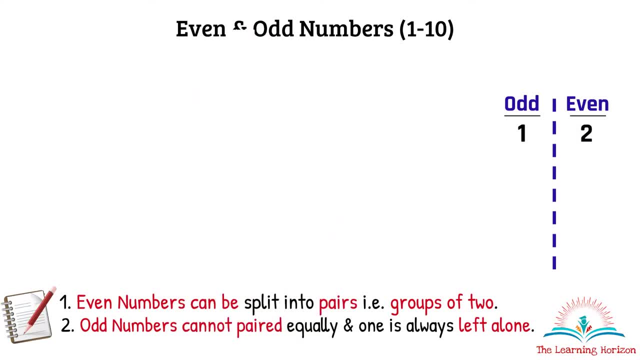 2 is an even number. let's look at next number, that is 3. here we have 3 tigers. let us split them into groups of 2. again, this tiger is left alone, so 3 is an odd number. let us look at number 4. we have 4 balls. we will create groups of 2, nothing left. so 4 is an even. 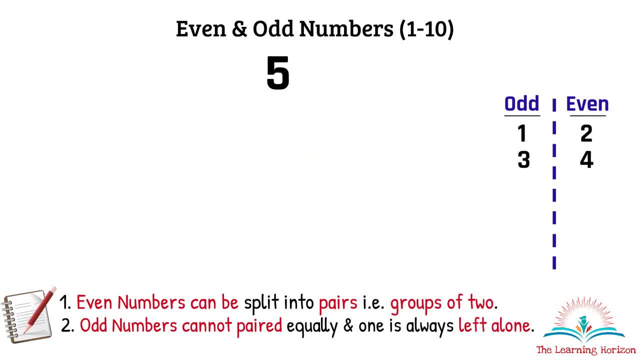 number number 5: we have 5 dogs here. group them into 2s, 1 left alone, so 5 is an odd number. number 6, that is, we have 6 flowers. again group them into 2s, nothing left, so 6 is an even. 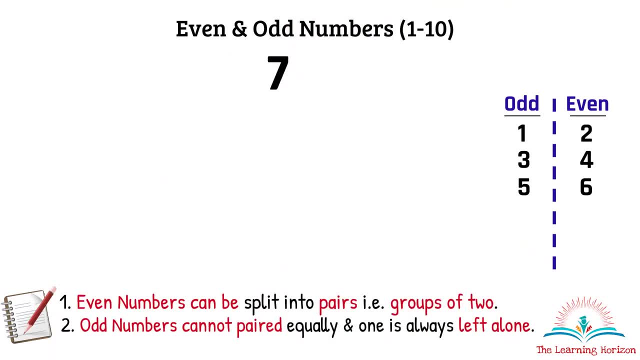 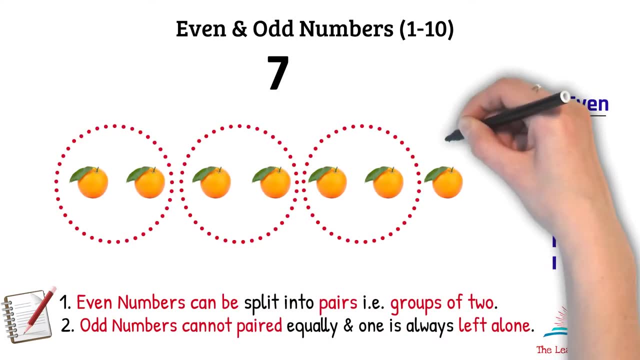 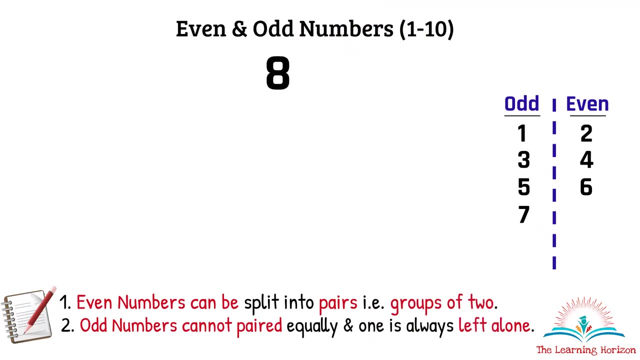 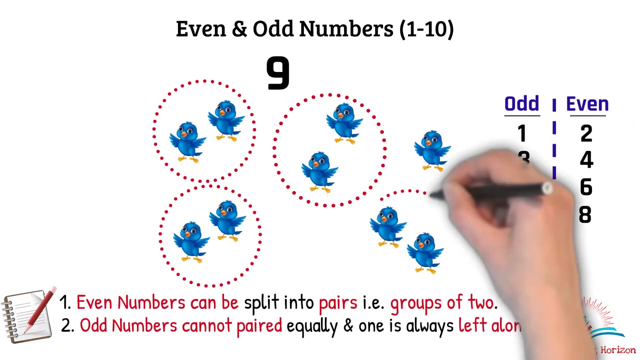 number number 7: we have 7 oranges here again. group them into 2s: 1 is left alone, so 7 is an odd number. number 8: 8: butterflies: groups of 2: nothing left, so 8 is an even number. number 9: 9: birds: groups of 2: 1 left, so 9 is an odd number. 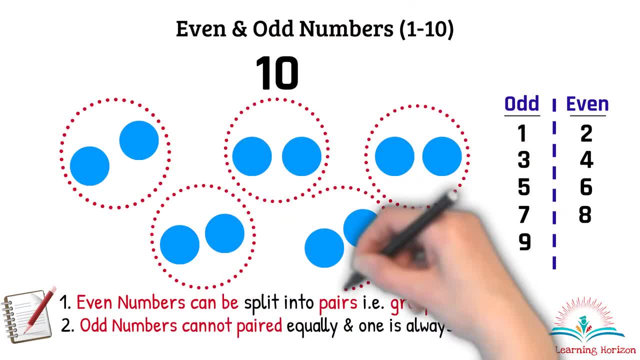 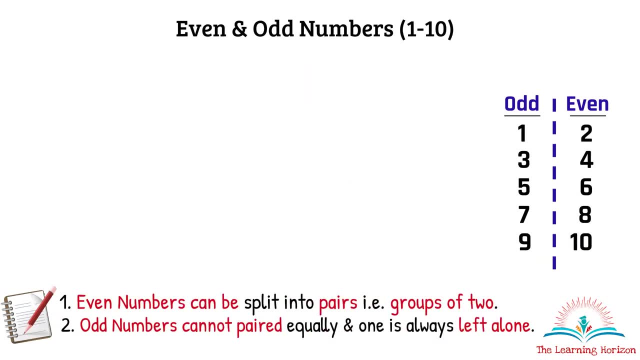 10 dots groups of 2, nothing left. so 10 is an even number. so 1,, 3,, 5,, 7 and 9 are all odd numbers, because when we split them into groups of 2, 1 is always left alone. 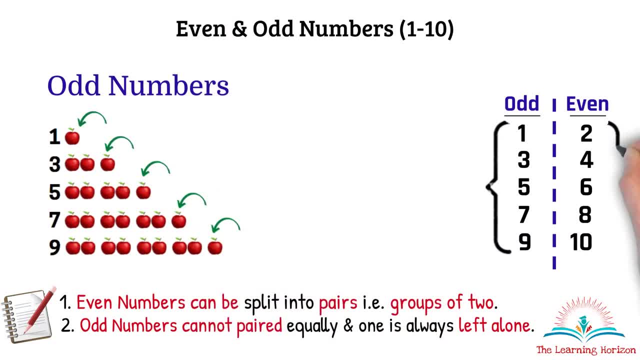 2,, 4,, 6, 8 and 10 are all even numbers because they all can be split into exact groups of 2,. we have seen how we identify if a number is odd, or even for numbers 1 to 10, now let 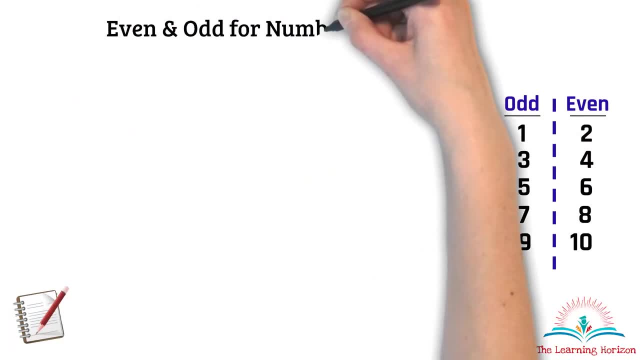 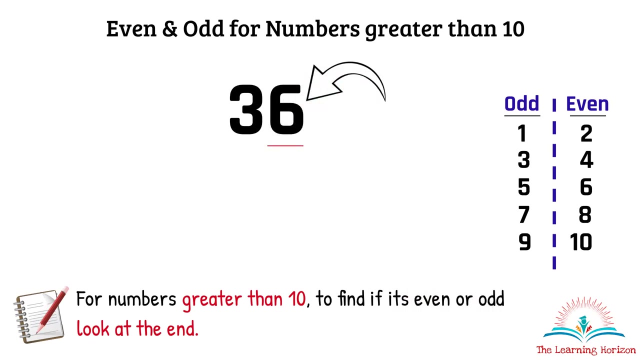 us see for the numbers that are greater than 10, for numbers greater than 10, to find if it's an even number here. if it's not even, then let us have some examples, if it is odd, or even from the numbersев the end. Twenty-six is the number at the end, 6 is an even number. 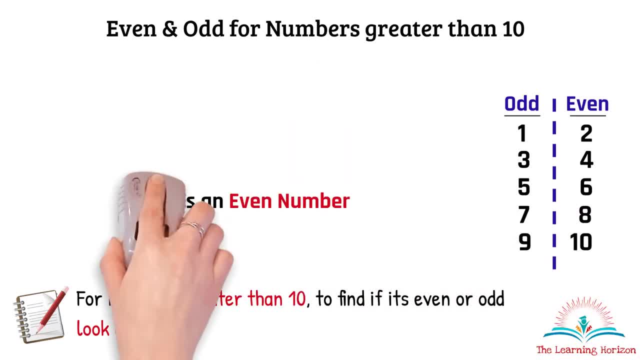 so 36 is an even number. let us look at some more examples here. 3 is the number at the end, 3 is an odd number, so 23 is an odd number. 8 is a richer number, zero is a more pathetic. 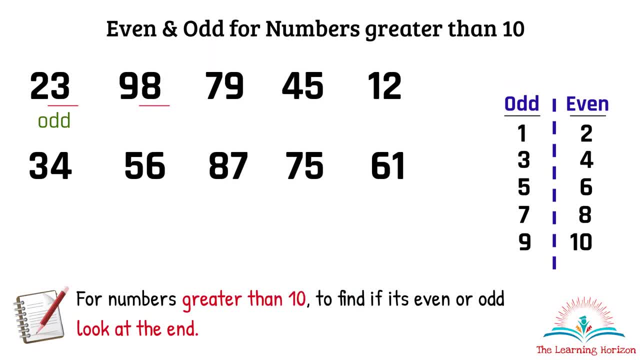 number an even number, So 98 is an even number. 9 is an odd number, So 79 is an odd number. 5 is an odd number, So 45 is an odd number. 2 is an even number, So 12 is an even number. 4 is an even. 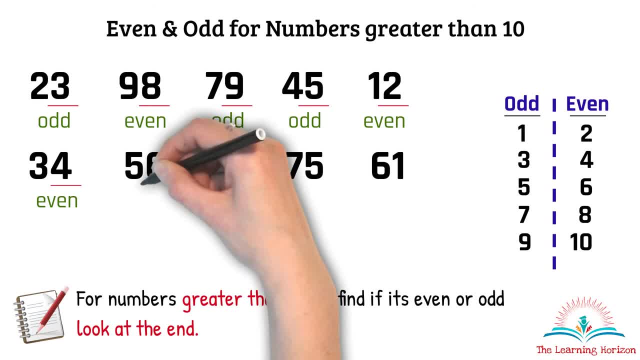 number, so 34 becomes even number. 6 is an even number, so 56 is an even number. 7 is an odd number, so 87 is an odd number. 5 is an odd number, so 75 is an odd number. 1 is: 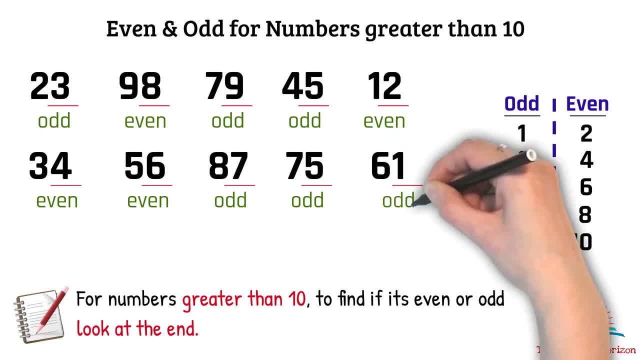 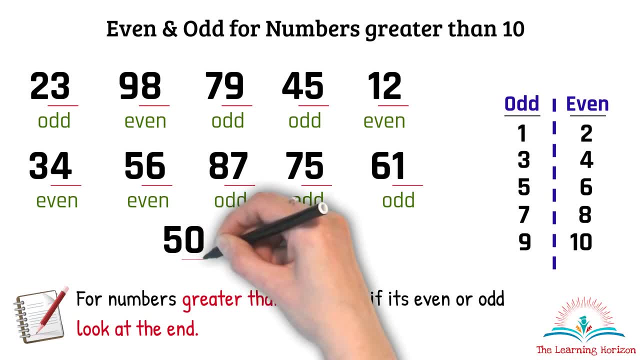 an odd number. so 61 is odd number. Now look at these numbers: 50 and 20.. They are both tens numbers. Since 10 is an even number, 50 and 20 are also even. So if a number ends with 0,, 2,, 4,, 6 and 8,, they are all even numbers. If a number ends with 1,, 2,, 3,, 4,, 5,, 6,, 7,, 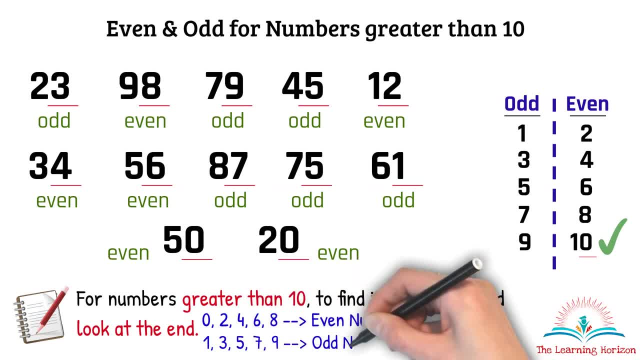 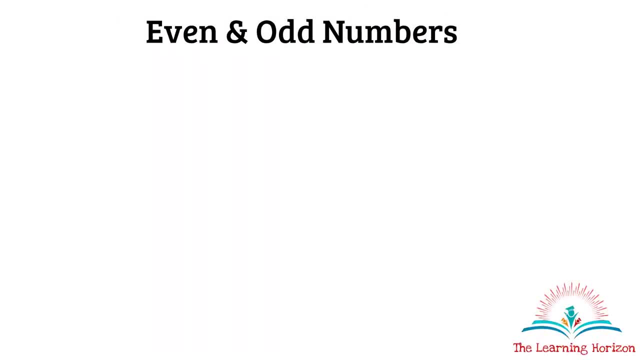 3,, 5,, 7 and 9.. It is an odd number, So let us now summarize: If you are an even number, you always have a pair. So if you look around, your friend will always be there. So 2,.